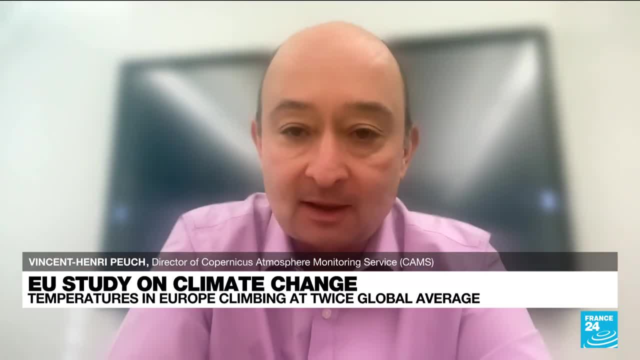 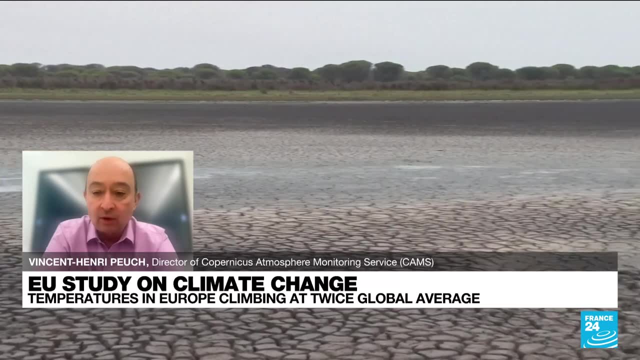 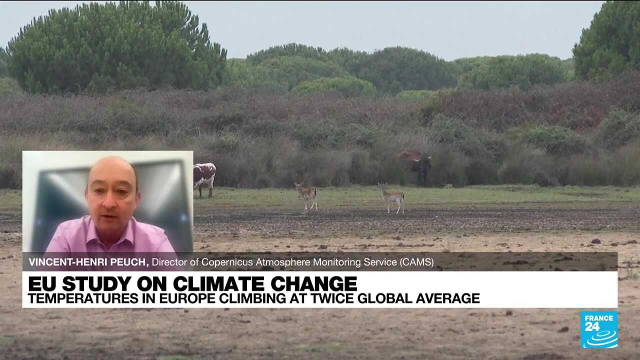 Yes. So what we observe is that Europe's temperature is increasing twice compared to the global average. There are two main reasons. The first one is that the European domain includes quite a number of high-latitude landmasses, like Greenland in particular. 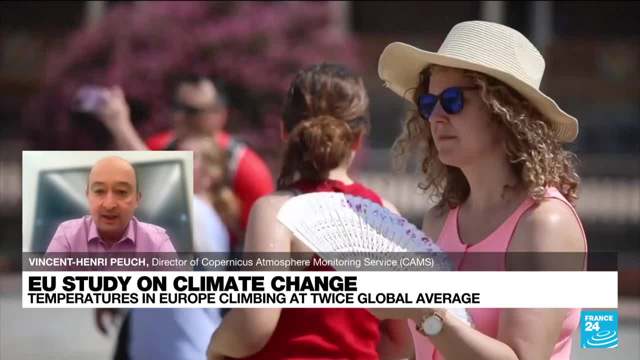 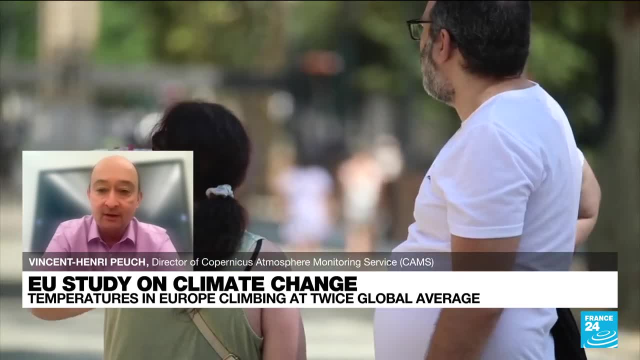 And what we know is that the and also sea ice in the Arctic. what we know is that with the diminishing of sea ice and the replacement of surfaces that reflect sunlight, there is an increase of temperature in high latitude. We call that Arctic. 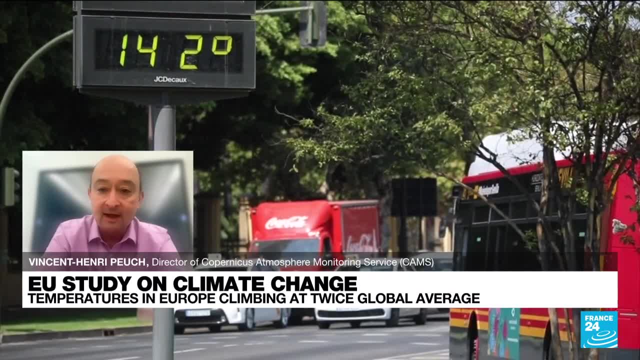 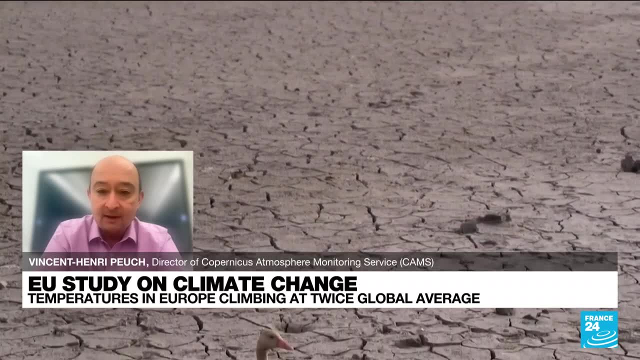 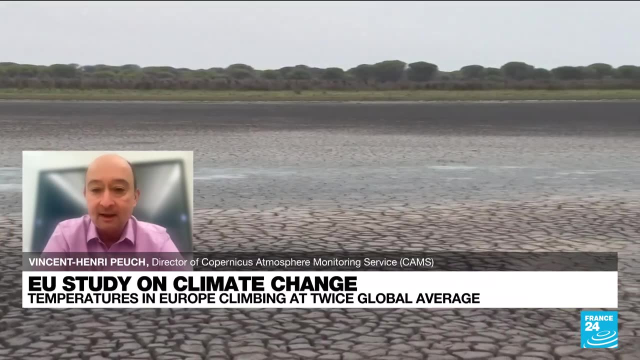 Arctic amplification And, as a matter of fact, we see that the high latitude increased temperature faster than the rest of the globe. The rest, why Europe is the temperature is increasing faster, is still a matter of question. What we see is that anticyclonic conditions are more frequent in the current decade. 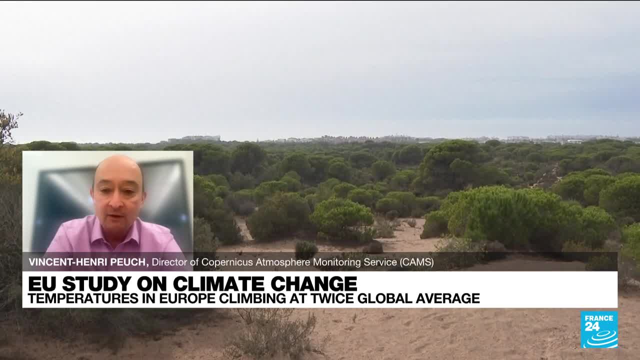 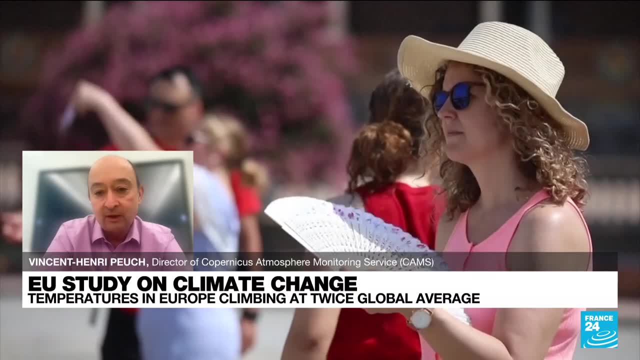 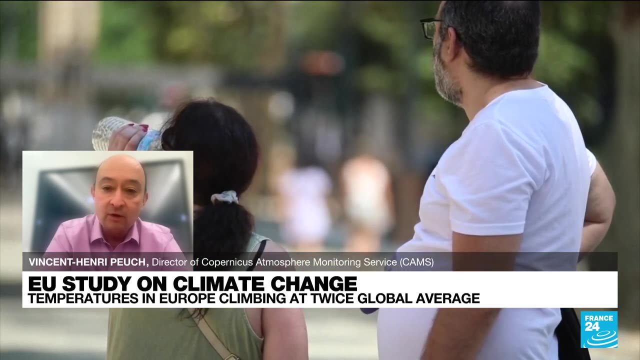 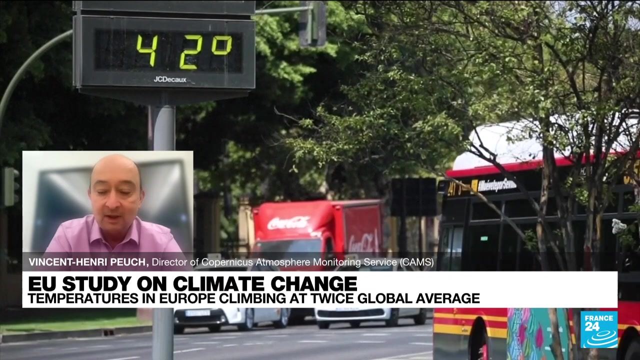 which means that there is a higher frequency of period of hot temperature, very stable weather. What we don't know exactly is whether it's a long-term trend and that we'll be there for a long time, or if it's a mode of variability of the weather and that for a number of years or a decade, will stay like this. 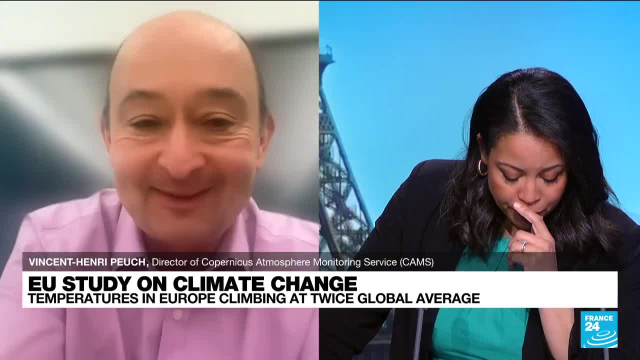 And then we'll. I mean that was going to be my next question, Vincent, because you made reference to the Arctic. this year, I mean it's important to say- experience its sixth warmest year on record. Greenland as well, having this kind of record. 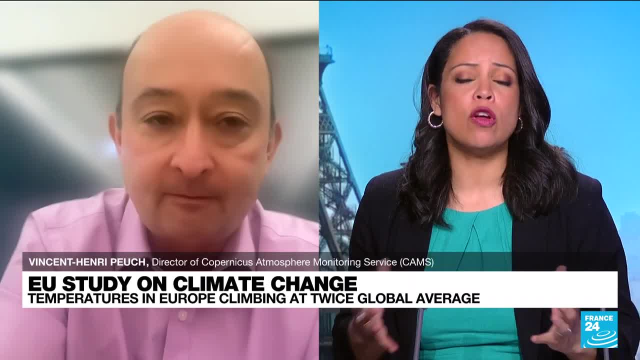 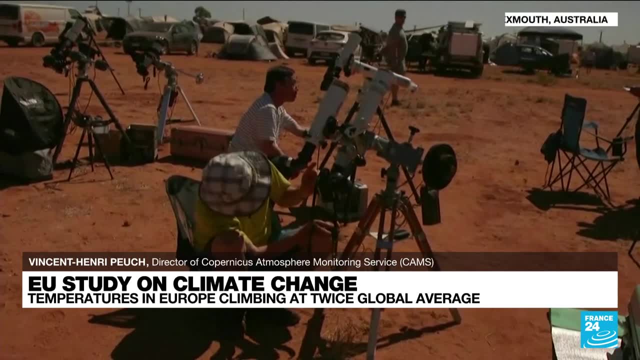 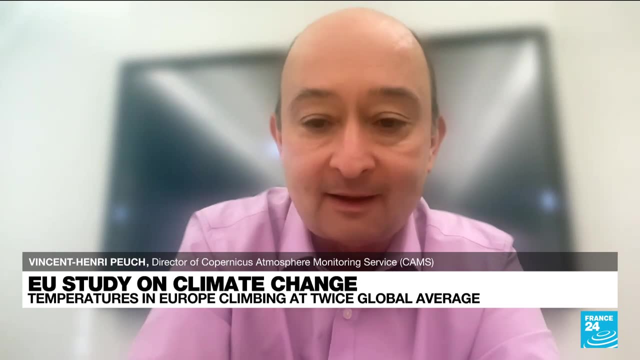 Breaking ice sheet melt. We still don't know whether these phenomenons are permanent or not. What we know is that, and what all the models and our data is showing, is that this is Sorry. No, that wasn't me, That was our background. 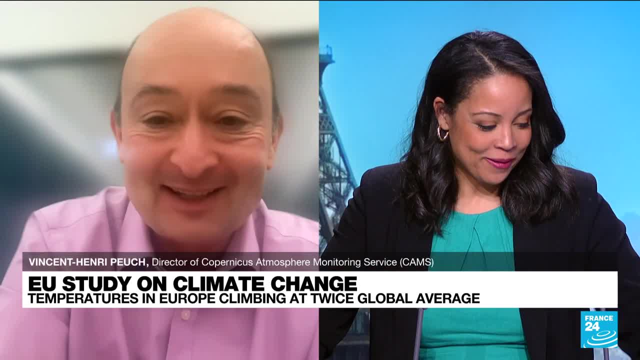 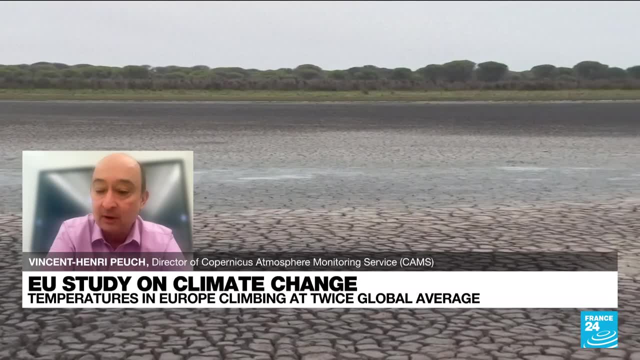 Our images that were making noise there. Go ahead, Vincent Henry. Yeah, So what we know is that there is a trend. There may be some variability from one year or another, But the model, The model of physics, the observation that we have, they all point in the same direction. 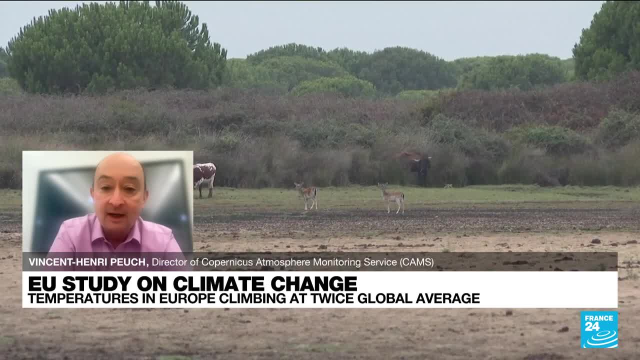 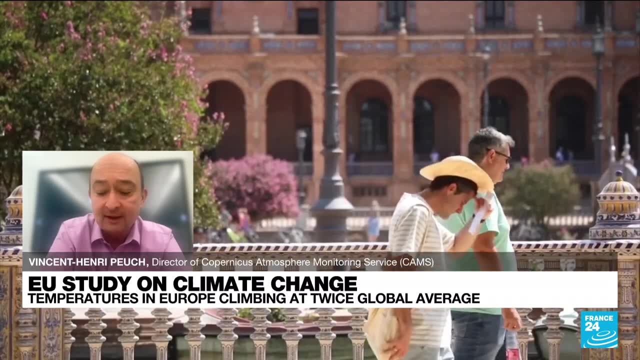 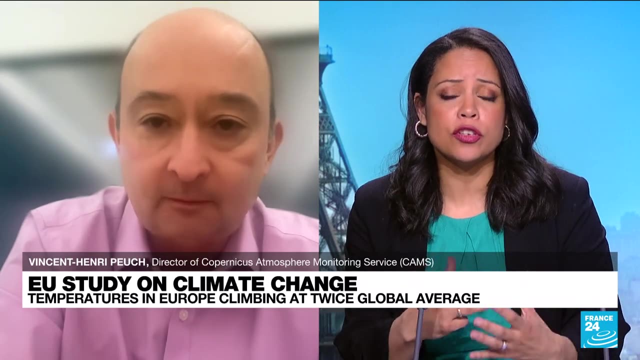 They all point in this direction of hotter weather and in the high latitude of reduction of sea ice and the cryosphere in general. So there is nothing like that. One of the things that your report talks about is the kind of hazardous conditions for human health with these extreme weather conditions. 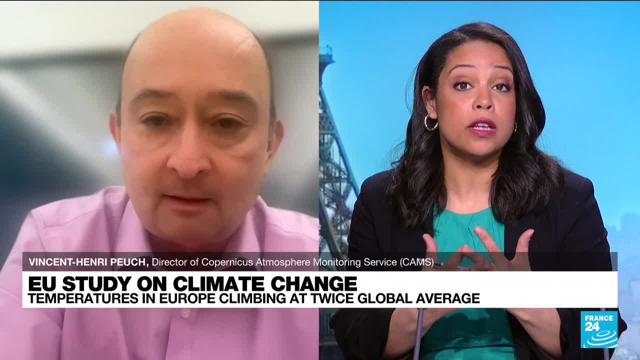 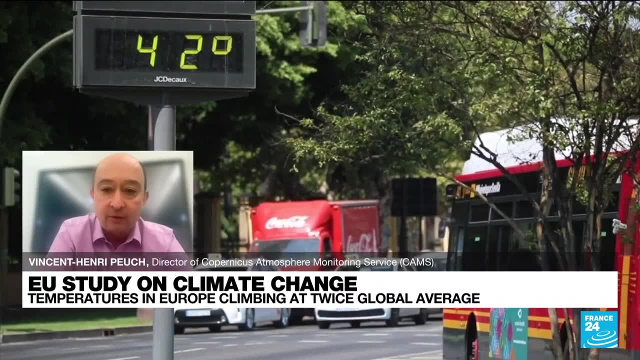 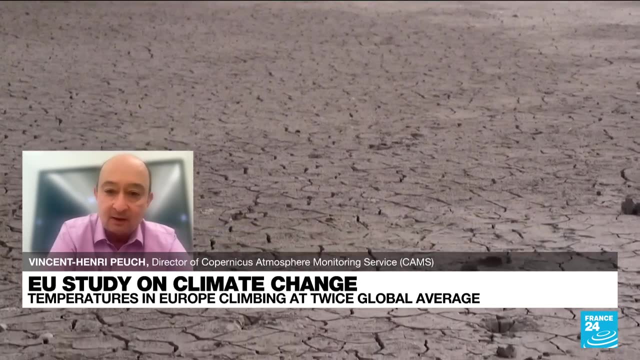 Walk us through some of the impact that these extreme weather conditions are likely to have on human beings. Yes, When we talk about One point, four degrees hotter summer is a bit abstract. What is maybe less abstract is to talk in terms of days with extreme heat stress. 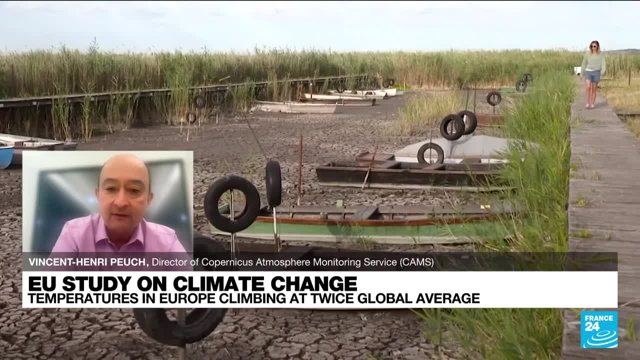 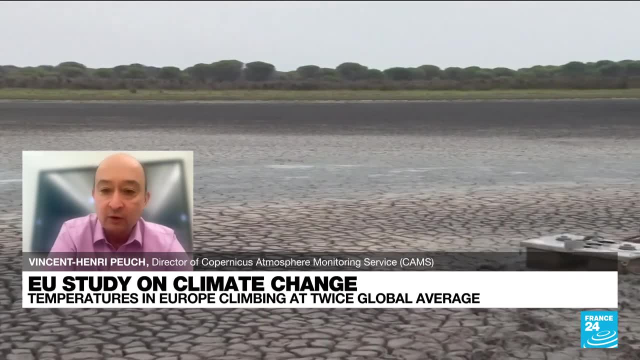 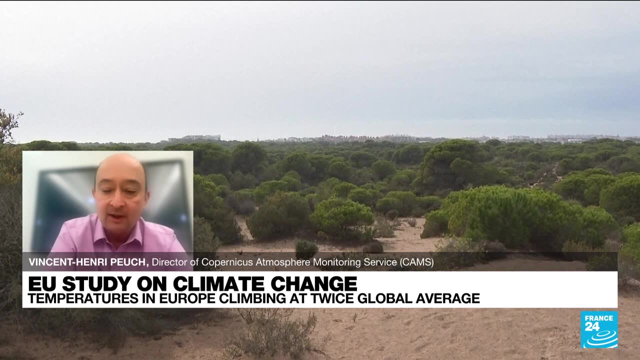 So the heat stress is an indicator which is defined by the way human bodies react to temperature, So it's calculated from temperature, but not only wind humidity, And when this index goes beyond a certain value it's called extreme heat stress And it leads to premature death in particular. 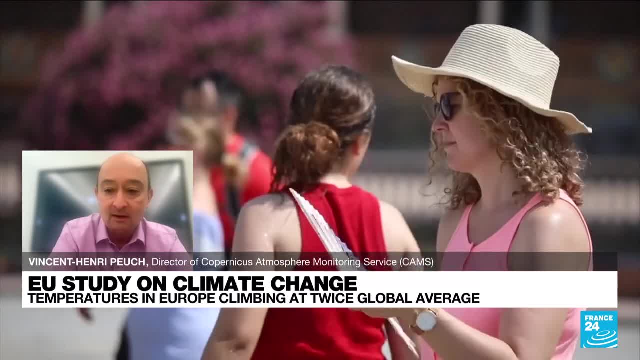 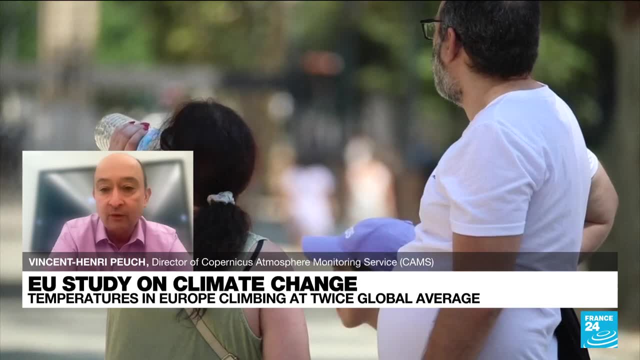 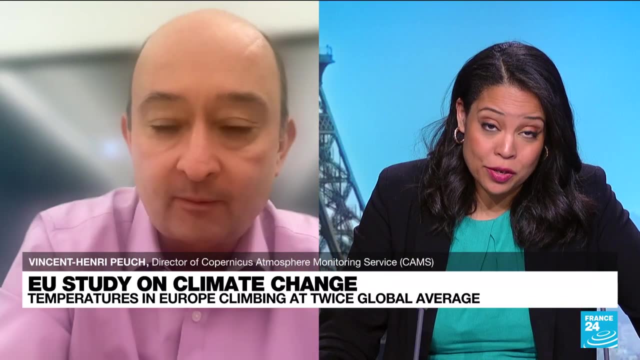 And what we've seen is that the number of these extreme heat days has been recorded last year Over many parts of Europe, south of Europe, it's over two months of extreme heat days that have been observed, I mean. so these conditions, or hazardous conditions, could be very dangerous indeed for human beings. 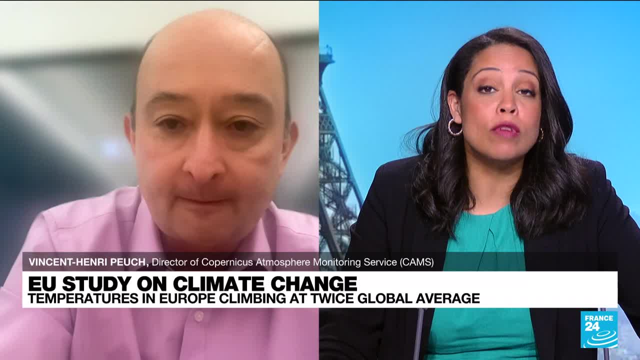 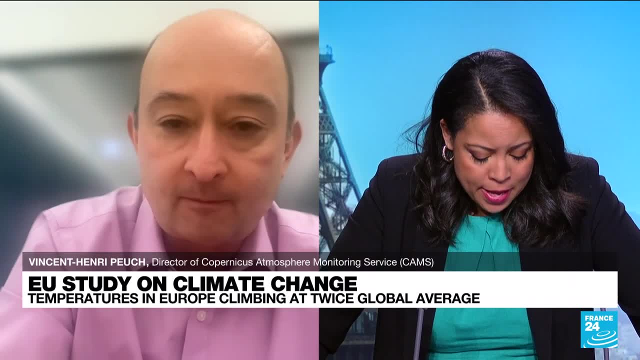 I mean UN- scientists have said that the planet has already warmed. It's warmed by 1.2 degrees Celsius. Where does that leave, Vincent Henry? the Paris Climate Accord, for example, in 2015,, where the aim was to kind of stay below 1.5 degrees Celsius? 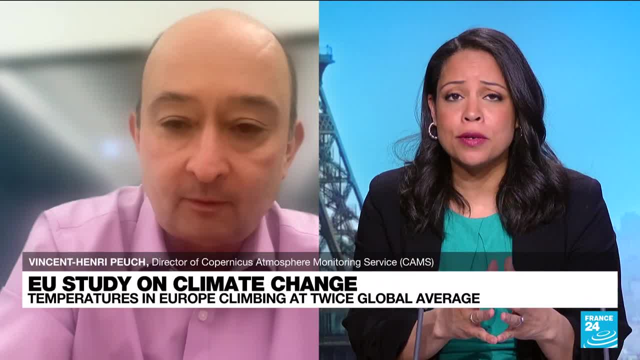 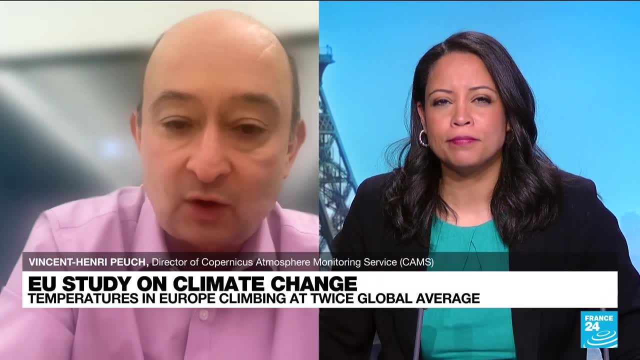 I mean, we're not so far off that temperature. Is it time to scrap that agreement, or start again, or ask for, you know, even further adjustments? What do you think? No, I think it's time to make things happen, maybe faster. 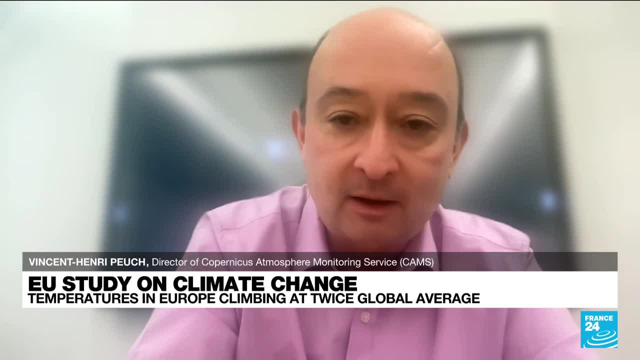 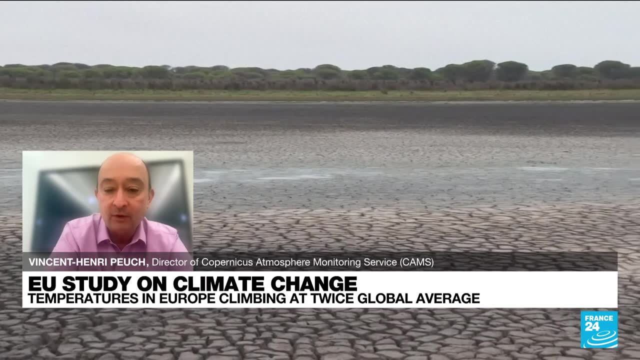 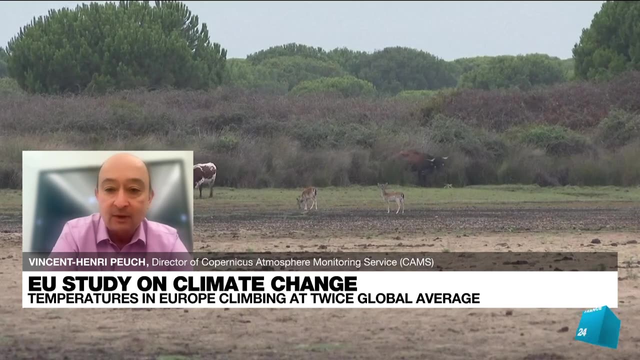 The problem is very simple. We still send emission of greenhouse gases and CO2 in the atmosphere. If we talk about the European Union last year, basically we emitted as many grams of CO2 that was done in the past year, So we are still emitting a lot.